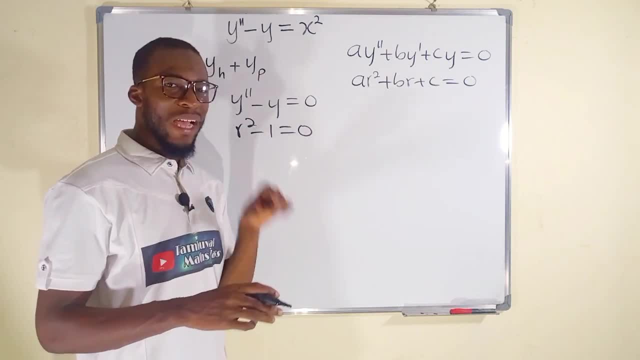 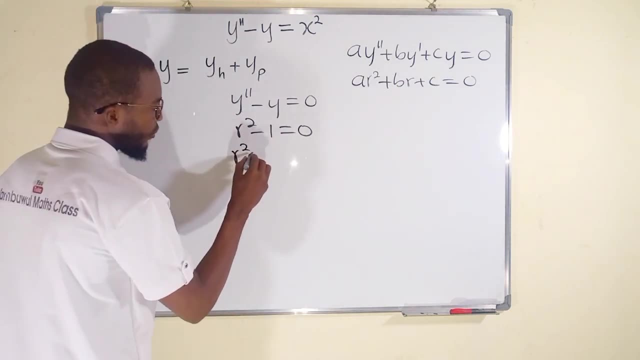 solve for the roots of the equation, and the nature of the roots will determine the form of general equation we are going to obtain. So now let us solve this. one r squared will be equal to positive 1 if you take negative 1 to the right. 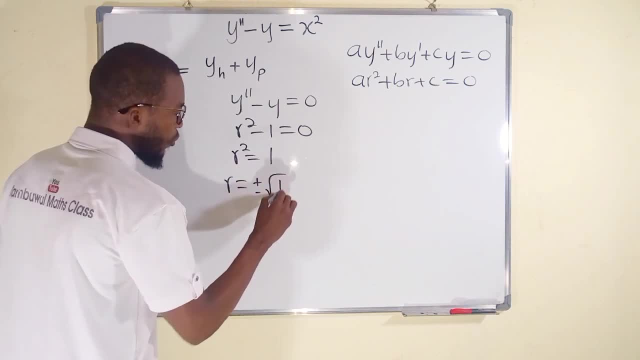 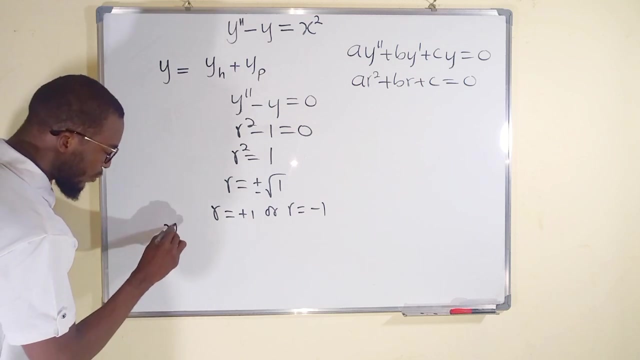 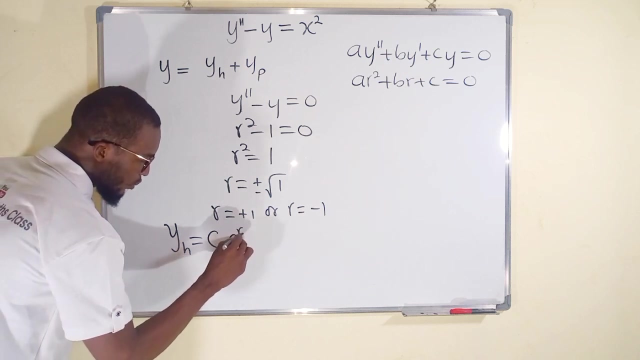 And r will be equal to plus or minus square root of 1. Therefore, r could either be positive 1, or r equal to zero negative one. so you can see we have real and distinct roots. so therefore, the general solution will be of this form: constant e to the first root times x, plus another constant e to the second root. 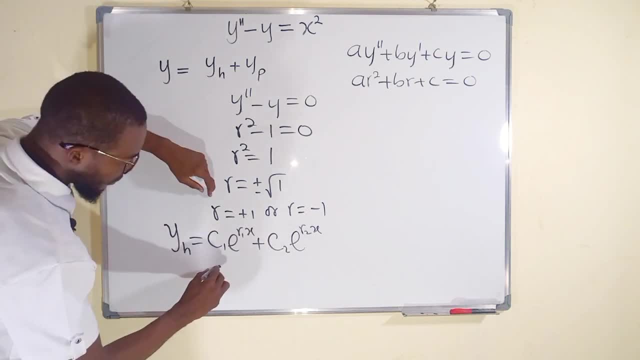 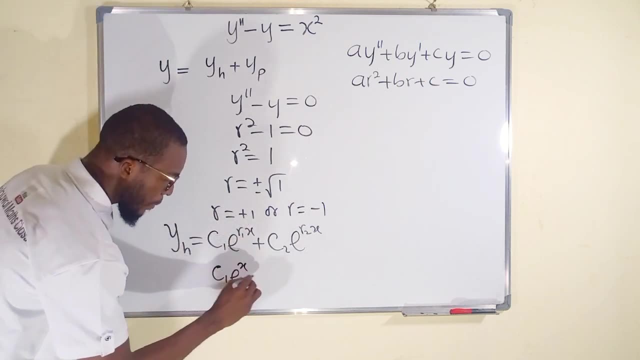 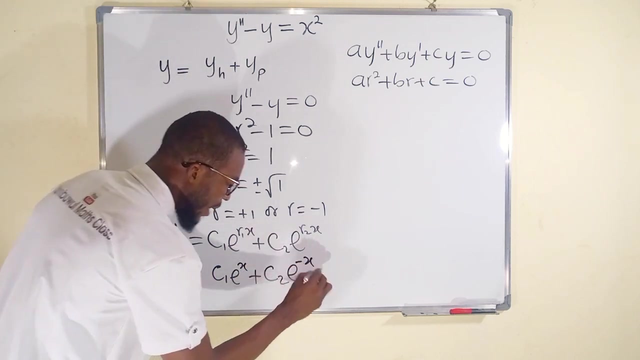 multiplied by x. so let's start. you can see that we have constant here. e to the first root- the first root is 1 times x is x plus c 2. e to the second root, which is negative: 1 times x is negative x. so this is the general solution to this homogeneous differential equation where we can now 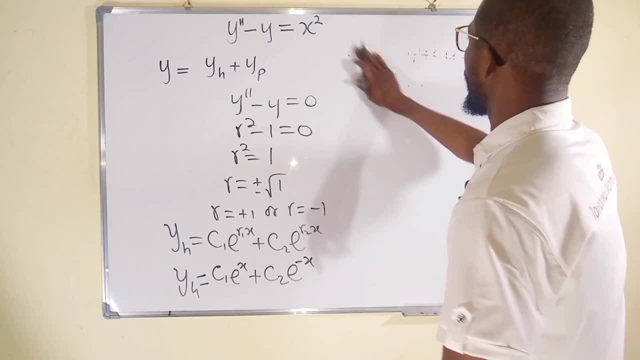 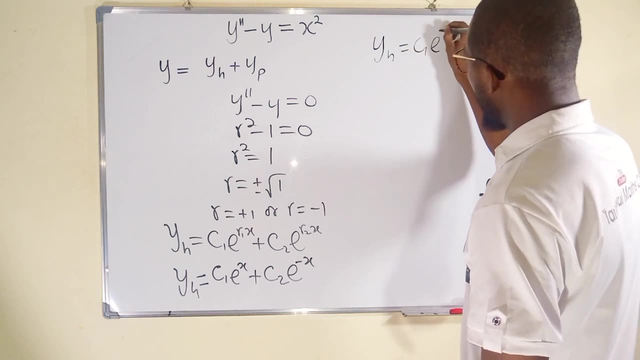 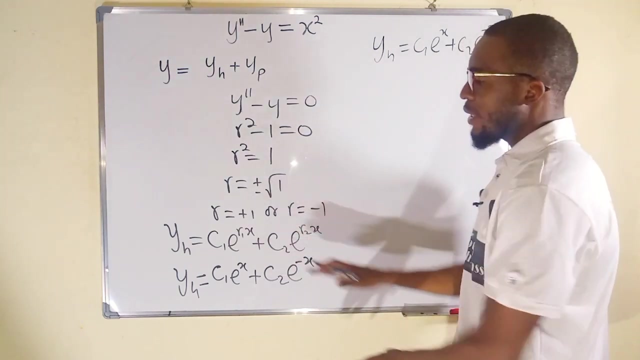 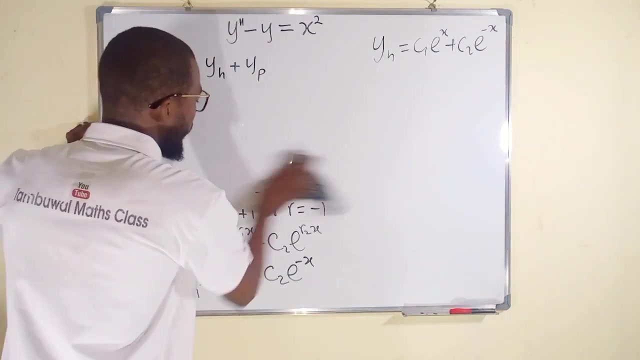 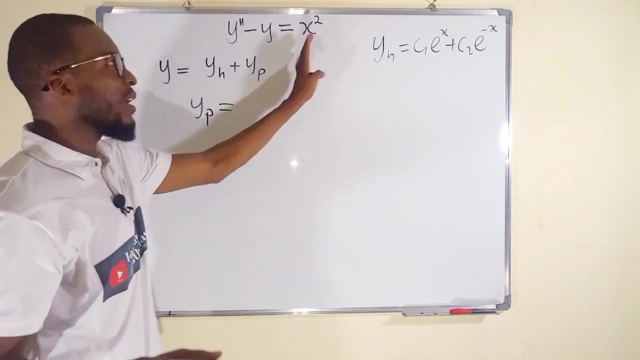 save this one for future use: y of h equal to c 1, e to the x plus c, 2, e to the negative x. so now let me wipe this one and find the solution to the other function, which is y of p. okay, now we want to find the solution to this y sub p. you know, it depends on the nature of the. 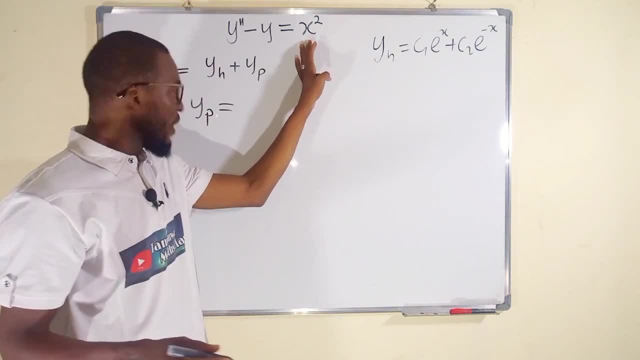 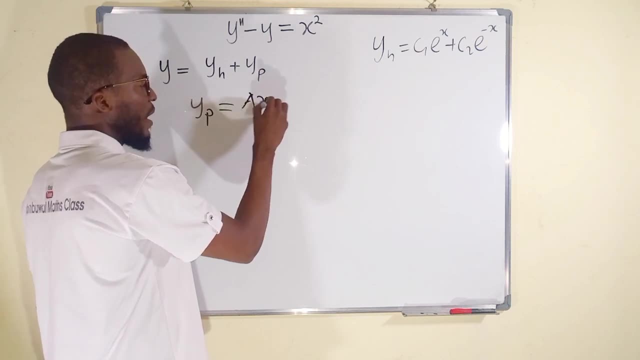 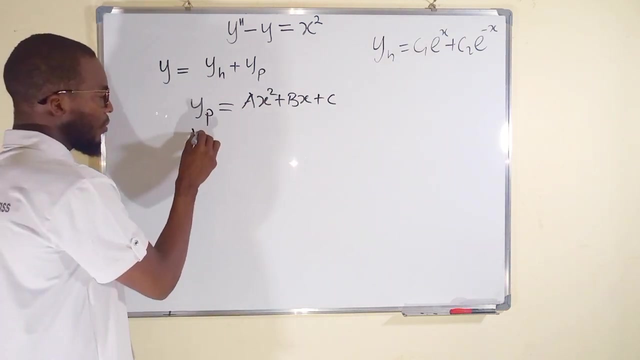 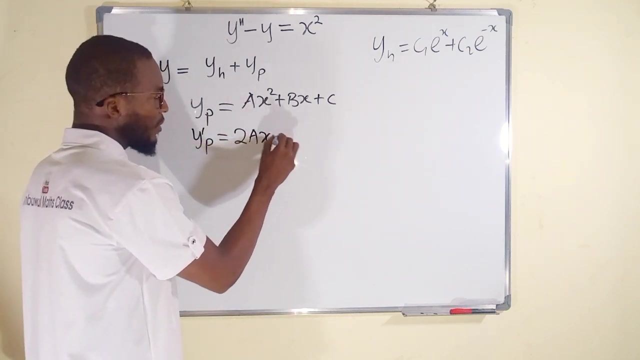 right hand side. if you have a quadratic function, then you set y sub p to be a quadratic polynomial. the general form is a, x squared plus b, x plus c. now you take the first derivative y prime of p equal to. if you differentiate the first time, you get 2a x. differentiate the second time, you get b. 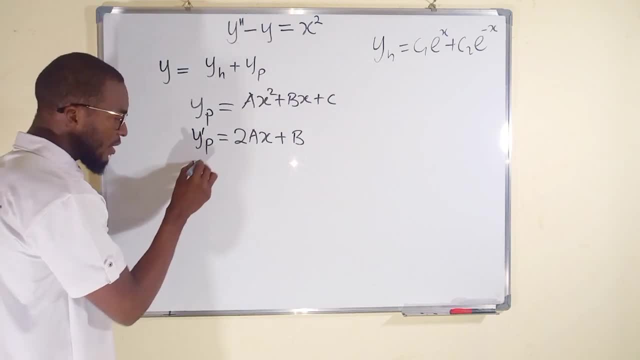 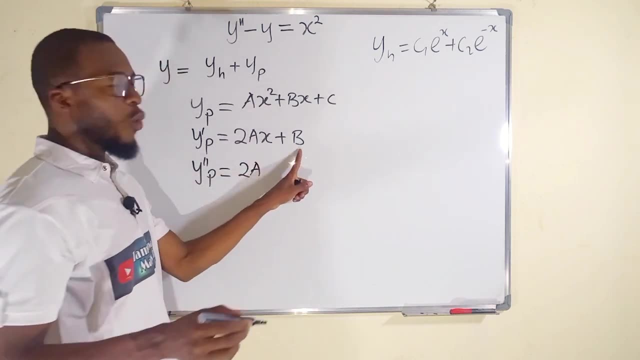 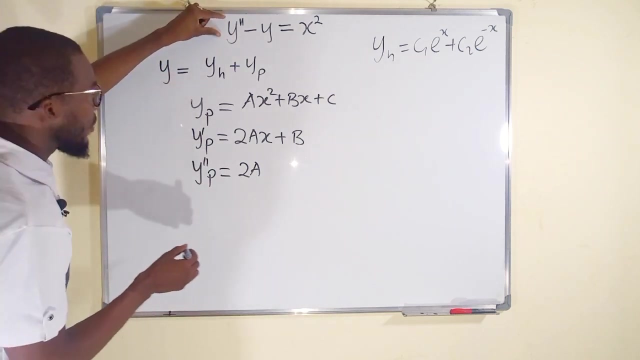 last one is constant, it becomes zero. you differentiate again the second time. differentiating this x will go, leaving 2a. and this is constant: it becomes zero. so we are going to substitute these three information in the general equation. y double prime should be replaced with 2a. 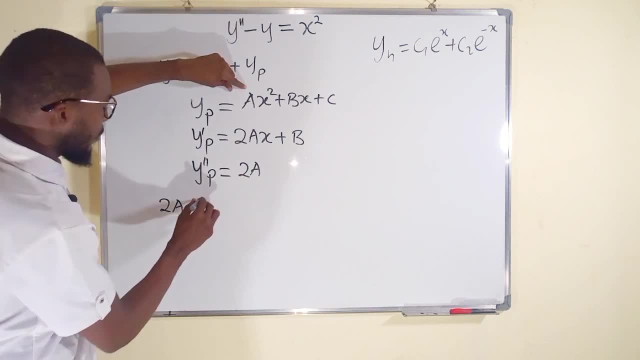 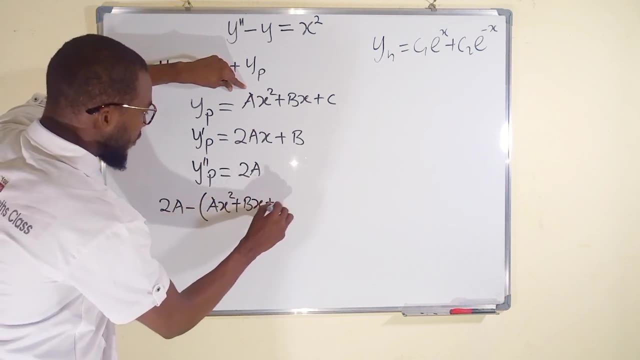 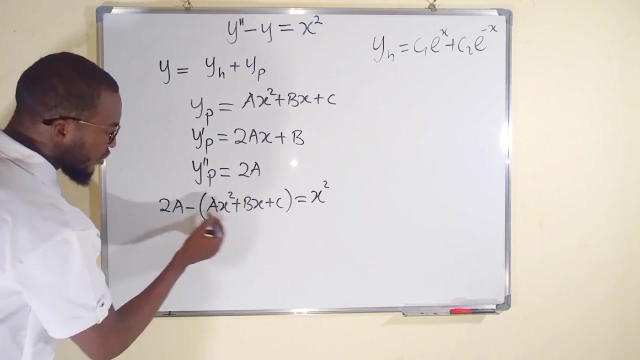 under minus y and you can see this is y. we put bracket, we'll write the y: a, x squared plus b, x plus c, and we set everything to be equal to the right hand side, which is x squared. now let us distribute negative sign. we have 2b, 12a, 2a, 2b, cube, 2a, 2b, cube, 2a, 2a. but let me bring those constant together. 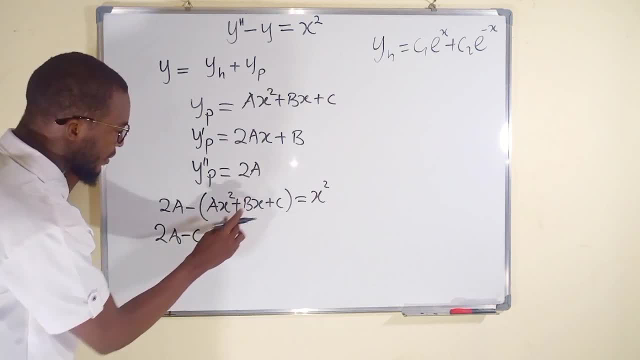 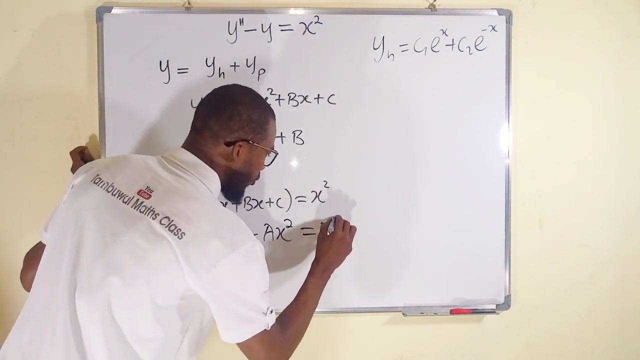 you can see i have only single constant here, so i have minus c, then followed by those with x. i have minus the x, the last one, those with x squared. i have only single term, minus a x squared. So we are going to solve this problem by relating the coefficients. 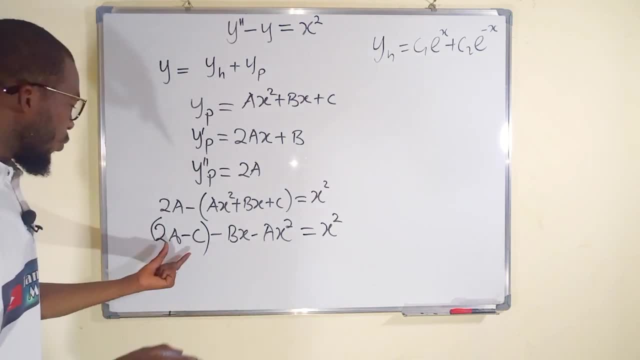 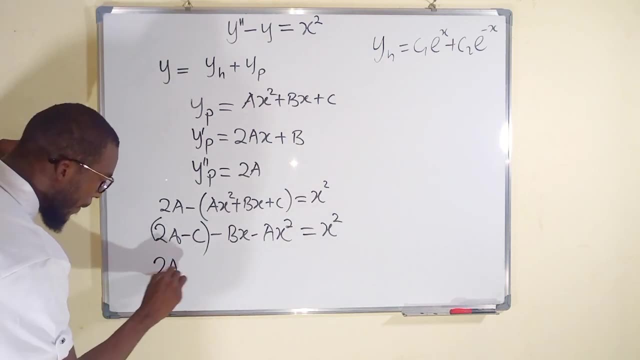 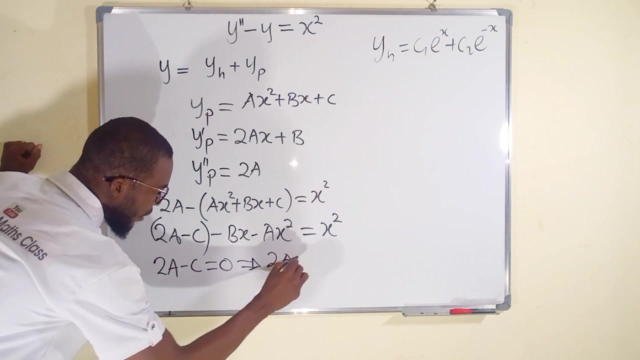 These are constant, remember So the constant. we don't have any constant to the right, So we are going to set the constant to be equal to zero. 2a minus c, equal to zero. This implies that 2a is equal to c. 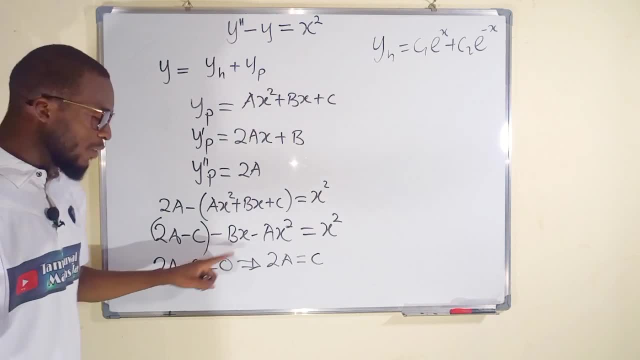 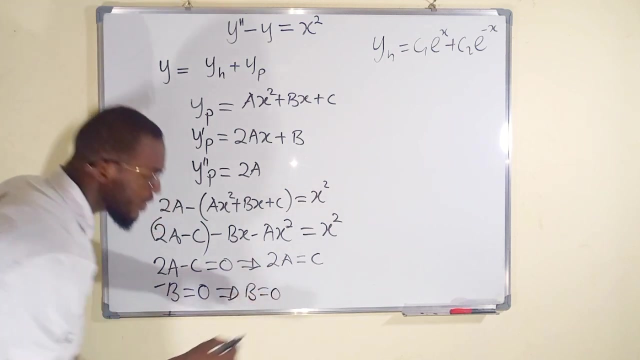 Then the coefficient of x to the left is minus b. Minus b, equal to. To the right, we don't have any coefficient of x, So this becomes zero. This implies that b is equal to zero. We have already solved for b. 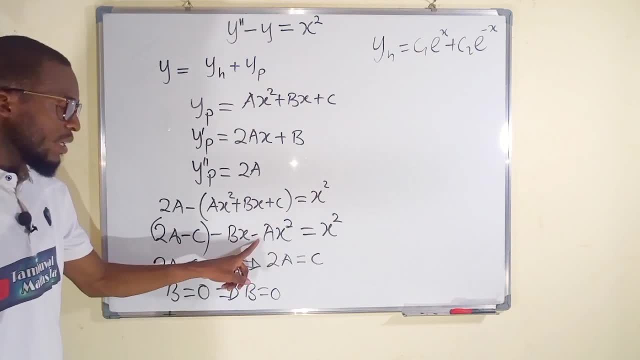 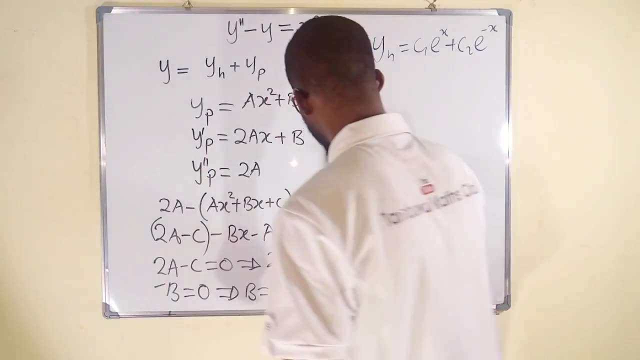 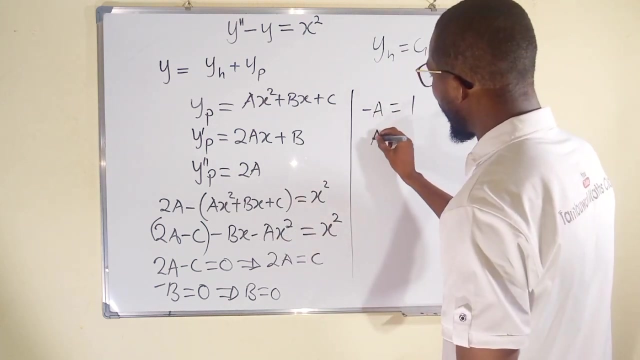 We have coefficient of x squared to be negative a to the left And to the right. we have the coefficient of x squared to be one. So let's come here. We have negative a To be equal to one. This implies that a is equal to negative one. 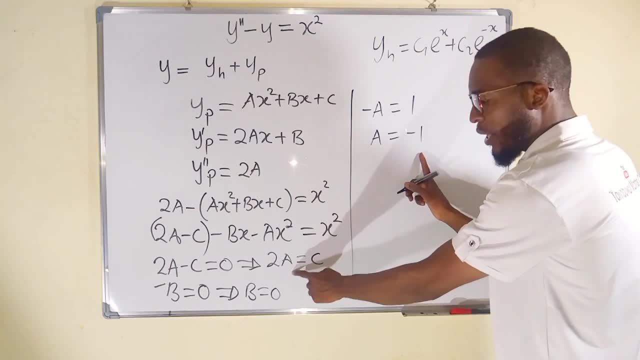 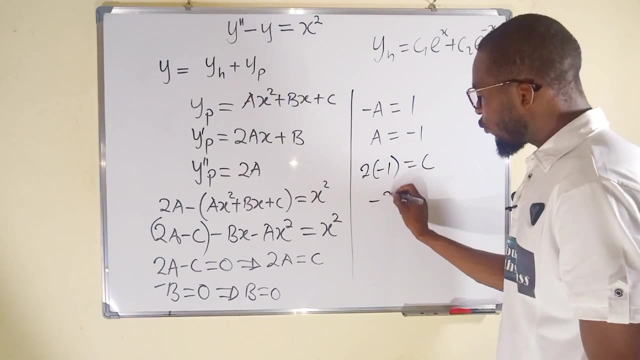 If a is negative one, we can solve for c here, Because 2a is equal to c. Therefore, 2 multiplied by negative one is equal to c Minus 2, because this time this is minus 2 equal to c. 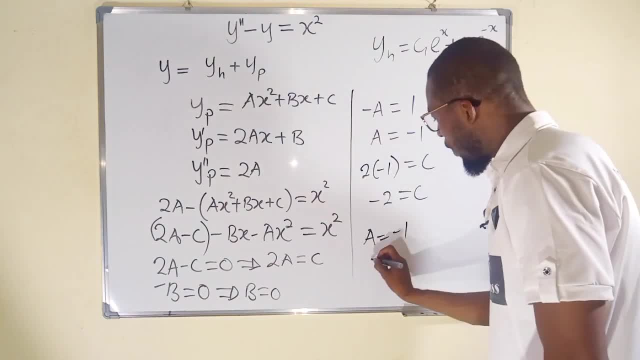 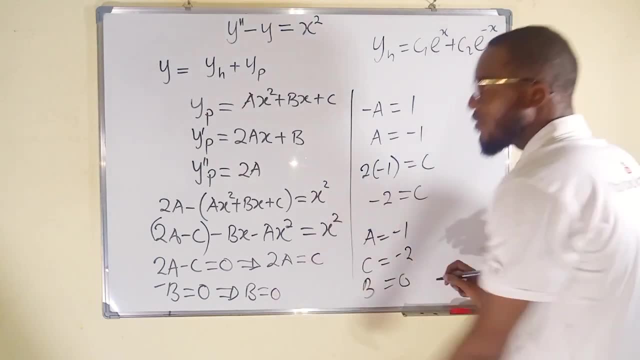 You can see that a is equal to negative one And c is equal to negative two, While b is equal to zero. You can see b is equal to zero. So now let us substitute a, b and c in y sub p here. 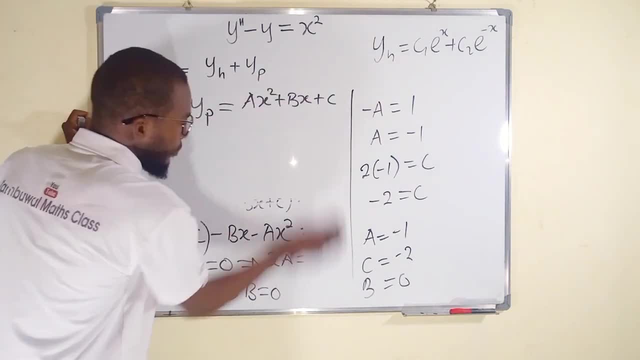 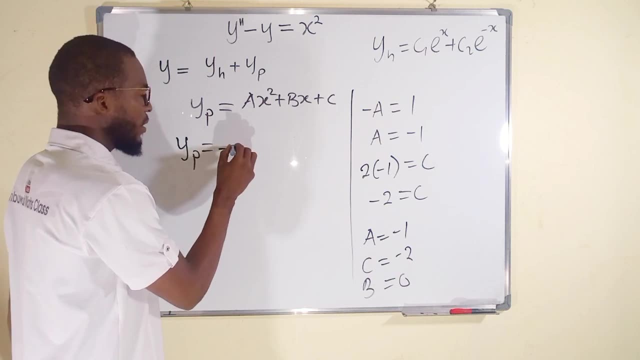 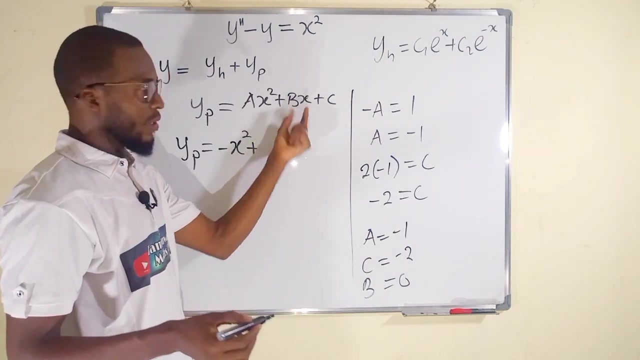 This is where we are going to substitute it. So y sub p equals a. We have it as negative one. So we have negative x squared Plus b is zero. So the whole of this time is gone. What we have left is c. 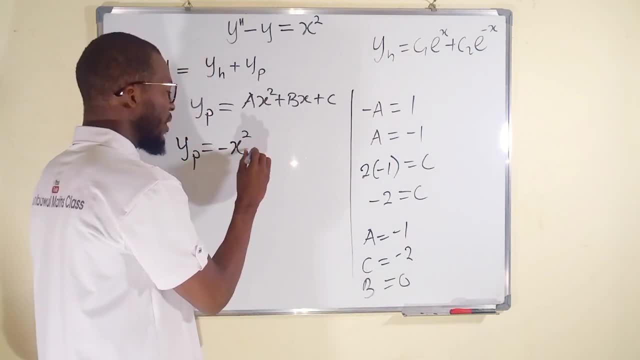 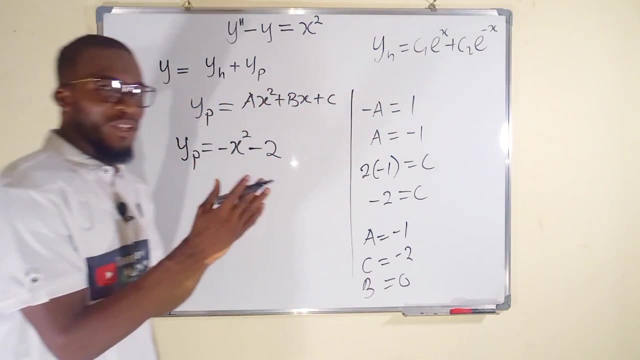 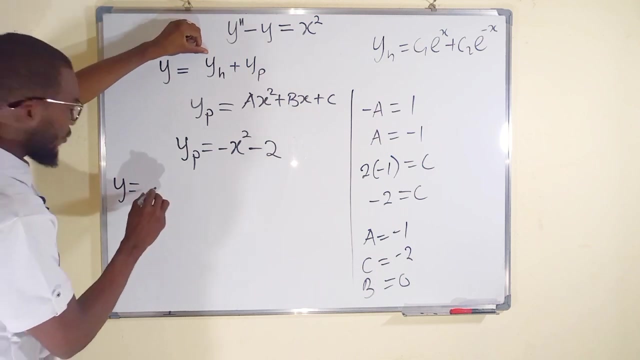 And c is negative two, So we have negative two. So we have y sub h and y sub p. Adding them together will give us the general solution to our equation. So y finally will be equal to y sub h, Which is c1 e to the x. 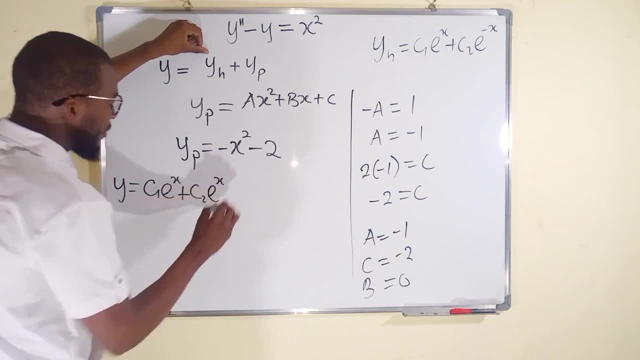 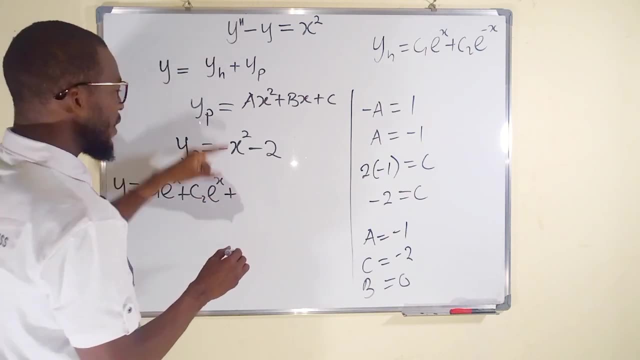 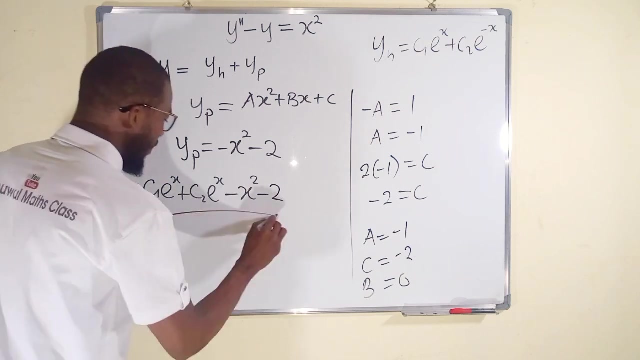 Plus c2 e to the negative x, We are done with y sub h. Then we add what we have as y sub p. This is negative x squared minus two. So this is the general solution to this equation here. But there is something I want us to confirm altogether. 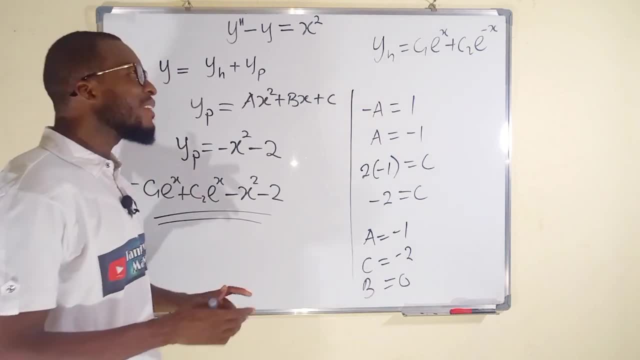 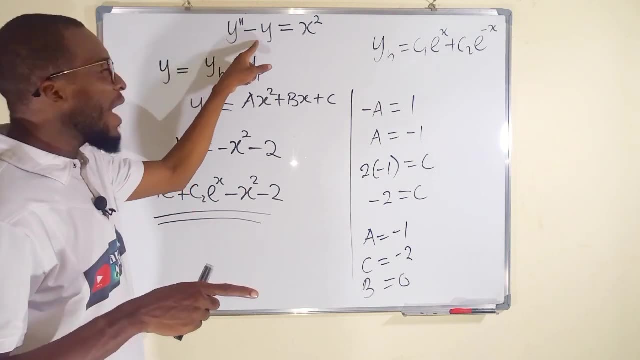 It is y sub p. We learned that y sub p is going to be a function which, when you take the second derivative of the function minus the original function, we are going to obtain x squared to the right. Let us see if this is true. 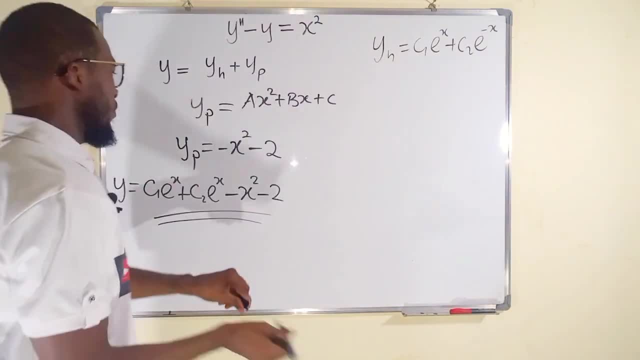 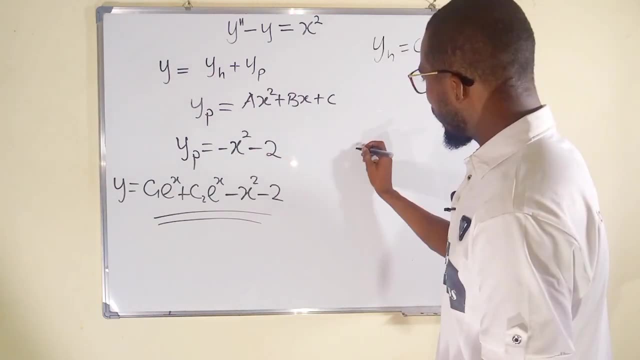 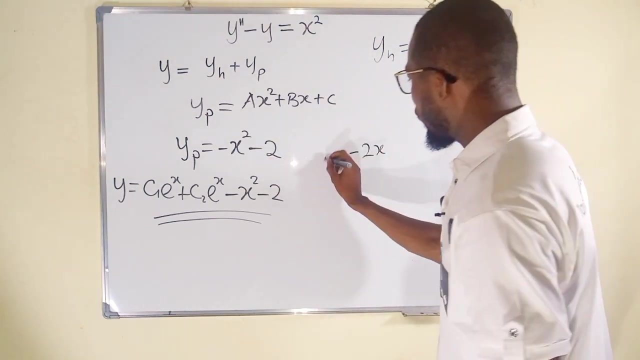 It is already done, So I just want to confirm it. This is y sub p. Let us take the first and second derivative of this. If you differentiate this, you get minus two x. then this becomes zero. So y prime of p is this. 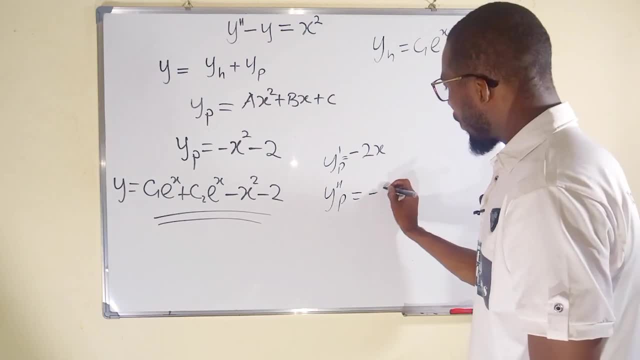 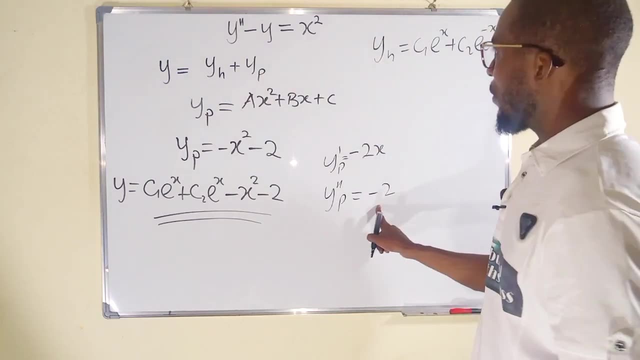 And y double prime of p will be equal to minus two. X will go. So now let us substitute it here to see whether we are going to get x squared. Y double prime is minus two, Then minus y. Y is minus x squared minus two. 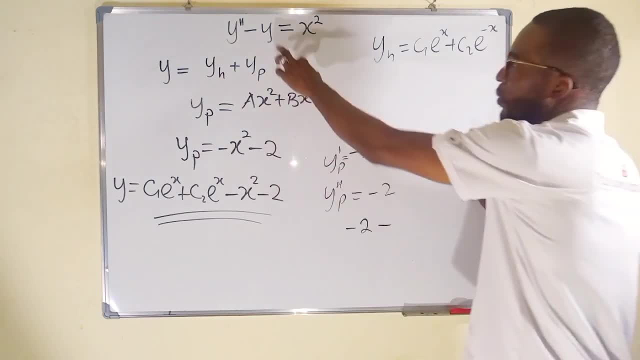 If you distribute this, you have minus two. Minus minus is plus x squared. Then this becomes positive two. You can see this. cancel this. What we have left is x squared. This is true To the right hand side. we have x squared. 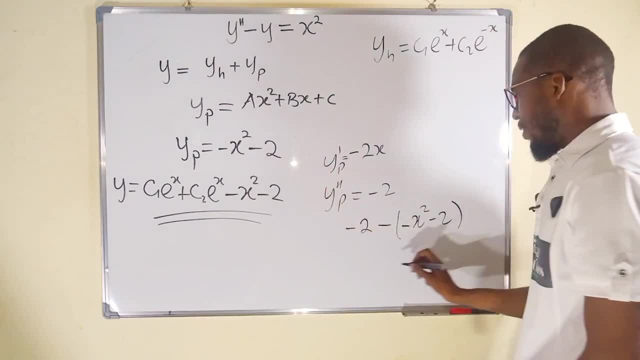 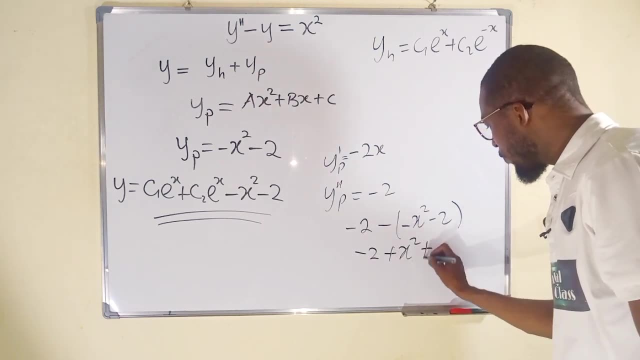 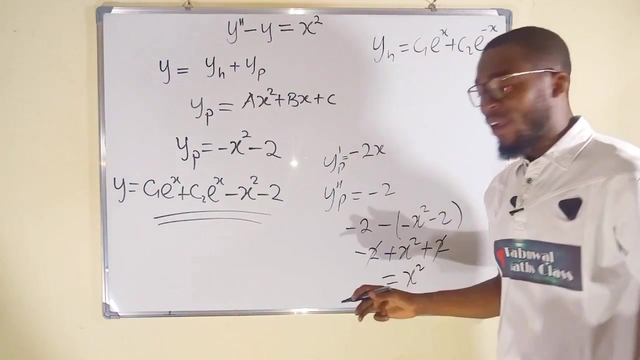